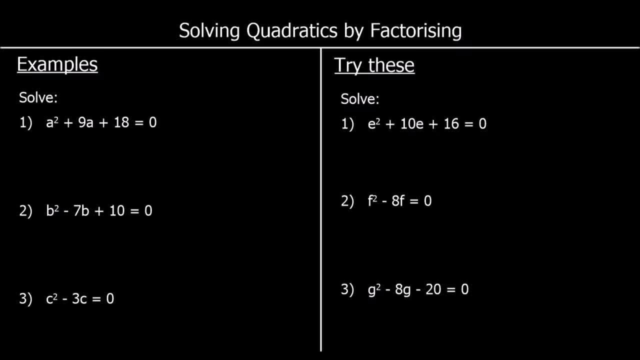 In these questions we are going to be solving quadratic equations by factorizing. So we know that these are quadratics because the highest power of the unknown is squared. So we've got a squared, b squared, c squared and so on. So that makes them a quadratic. 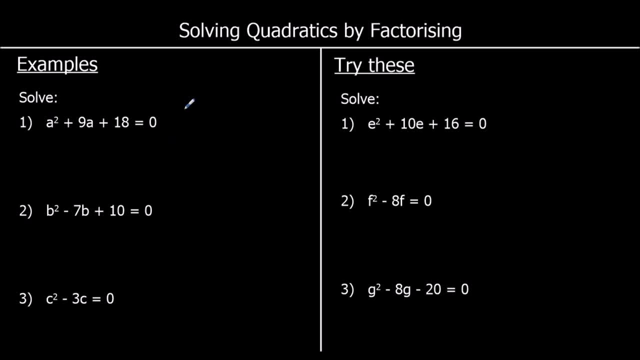 They're equations because they've got an equal sign, And to solve an equation that means we're finding out what the unknown is. So we're going to find out what a can be for the first one, what b can be for the second one, and so on, So we're going to solve them. 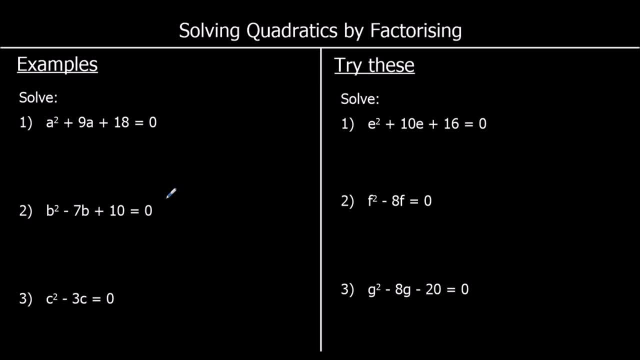 by factorizing, and that means putting them into brackets. For the first one, we're going to have double brackets And you should start to recognize this form. So it's a something squared. So we've got an? a squared term, then an? a squared term and then an? a squared term. 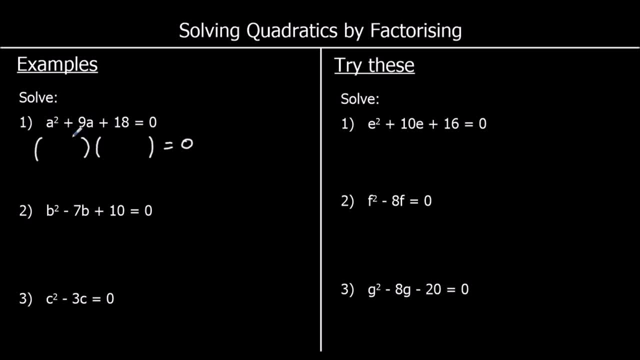 Then a number. This form goes into double brackets And we're going to have an a in both brackets because a times a is going to make a squared. Then we're going to look for two numbers that multiply to make 18 and add to make 9.. So we write down the factors. 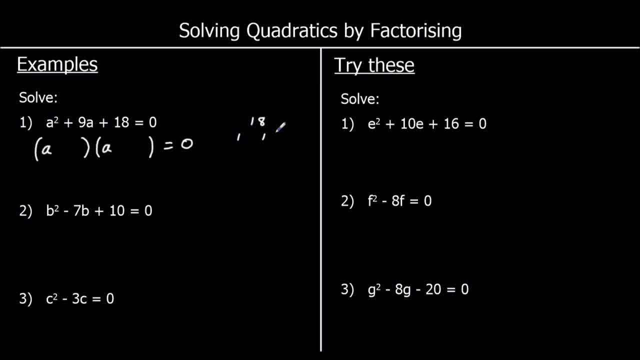 of 18.. So 18 is 1 times 18,, 2 times 9, and 3 times 6.. Which of these pairs can add to make 9?? That's 3 and 6.. And it's going to be a positive 3. 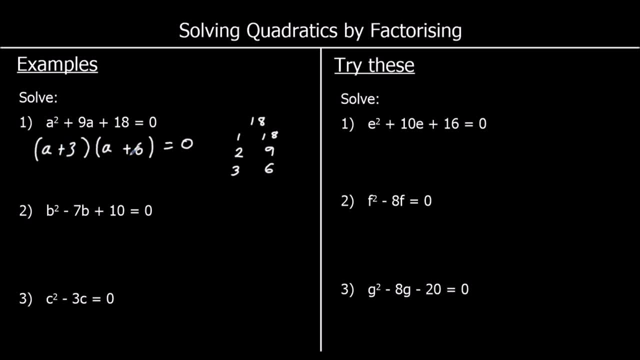 and a positive 6.. So 3 and 6 add to make 9 and multiply to make 18.. So if I expanded this bracket I would get a squared plus 9a plus 18.. So how can we solve it from here? 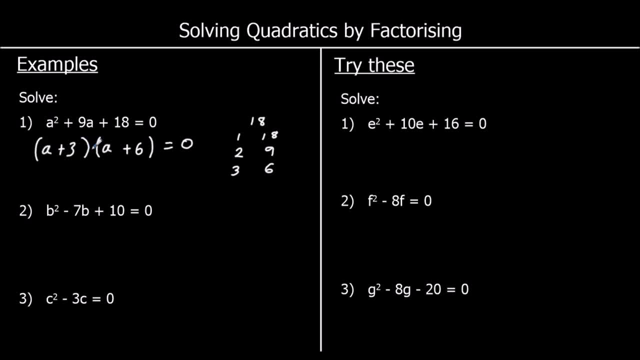 So this says: a plus 4a 3 times a plus 6 equals 0. And to equal 0, either this bracket, so either a plus 3 or a plus 6 must equal 0. Because 0 times something is 0. And something times 0 is 0. So what? 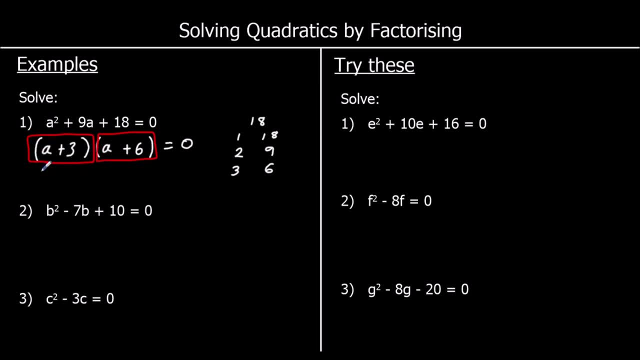 would make a plus 3, 0?. So what would make a plus 3, 0?? So what would make a plus 3, 0?? So for a plus 3 to equal 0, what is a a is going to be negative 3.. Negative: 3 plus 3. 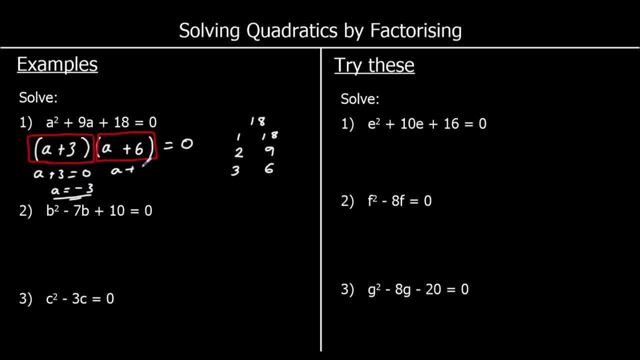 is 0. And for a plus 6 to equal 0,, a would have to be negative 6. Because negative 6 plus 6 is 0. So for our bracket, a plus 3, to make it 0,, it would be minus 3.. For a plus: 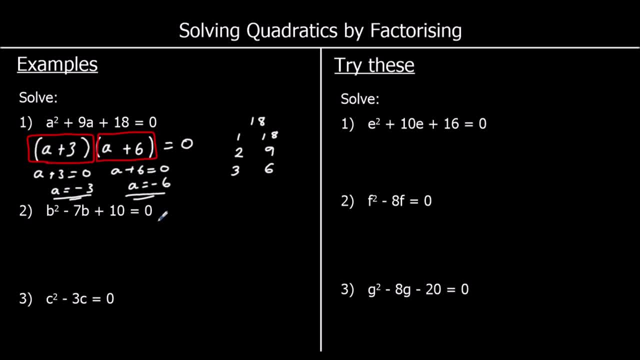 6 to equal 0,, it would be negative 6.. And for a plus 6 to equal 0, it would have to be 0, a would be minus 6.. So we've got two answers, And that is what we usually get for. 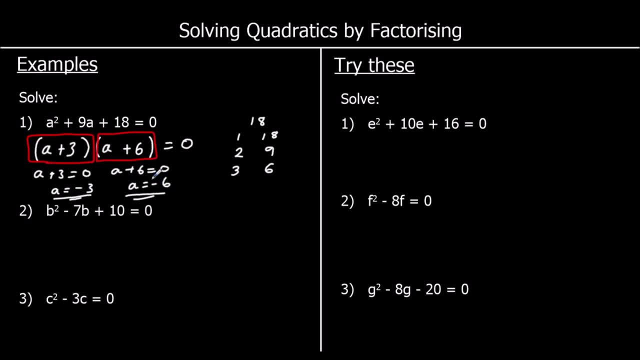 quadratics, We usually have two different answers. So we've got a can be negative 3, or it can be negative 6. And if we substituted either of them into the top we would get 0. So they are our answers For the second one, same again. So we've got our quadratic. 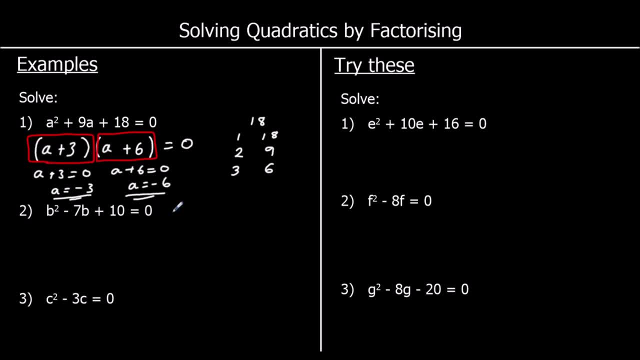 equation It's equal to 0.. 0, which it has to be for us to solve it. So we've got b in both brackets. We're going to put it into brackets. It's the same form: double brackets. We're looking for numbers. 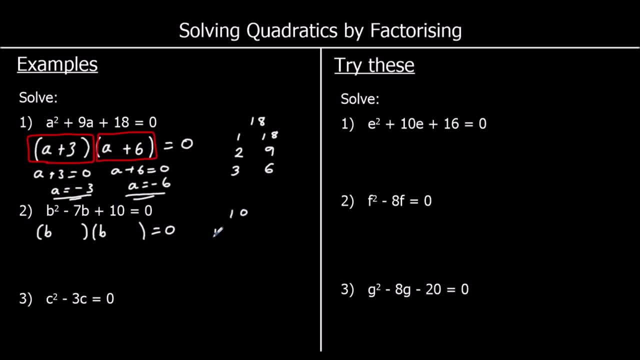 that multiply to make 10 this time, So 1 times 10, or 2 times 5.. We want to make a negative 7.. So that's going to be a negative 2 and a negative 5. They add: 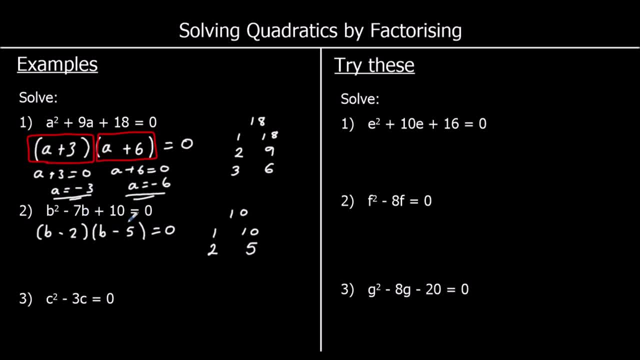 They add to make negative 7. And they multiply to make a positive 10.. So we know either b minus 2 is 0, or b minus 5 is 0. So if b minus 2 equals 0, b would. 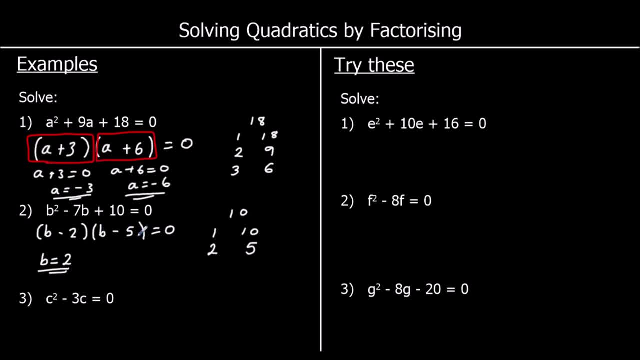 be positive 2.. And for b minus 5 to equal 0,, b would have to be 5.. 2 minus 2 is nothing and 5 minus 5 is nothing. So our answers: b can be 2 or 5.. Again, there are two answers. 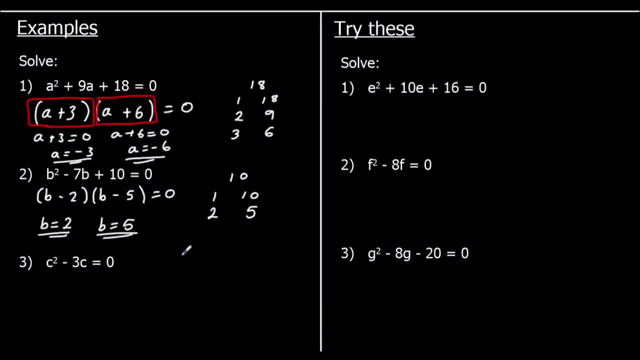 For number 3, we have a different form. This time we've got c squared minus 3c, So this is a single bracket factorizing. So this is going to go into one bracket. Usually if there's two terms, that means we've got one bracket. the exception is the difference of two squares. 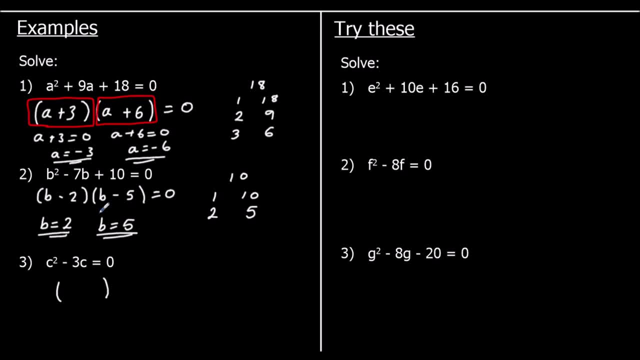 where we've got square numbers with a minus between them, so c squared minus 3c. so what can i take out of both of those terms? they've both got a c in them, so c can come outside the bracket. c times what would make c squared. that's c and c times what would make. 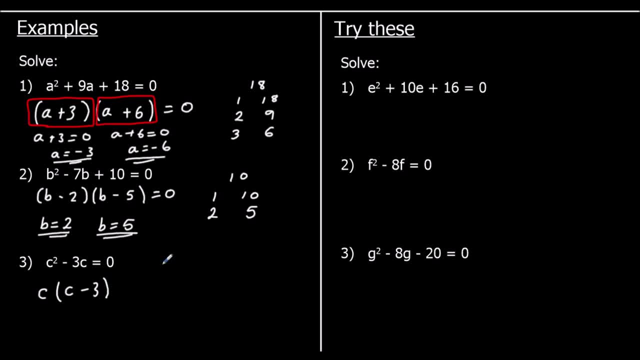 negative 3c, negative 3.. so this time we've still got two things multiplied together, so either c equals zero or c minus three equals zero. so for c to equal zero, well, c zero. so either c can be zero or c can be a positive three, because positive three minus three equals. 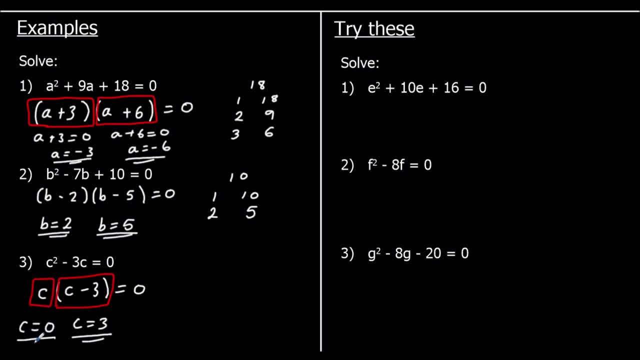 zero. so c can be zero or three. and again, if we substitute these in to the top to our question, we should get zero. so zero squared minus three zeros is zero. or three squared minus three, threes is zero. okay, three for you to try. so pause the video and give them a go. 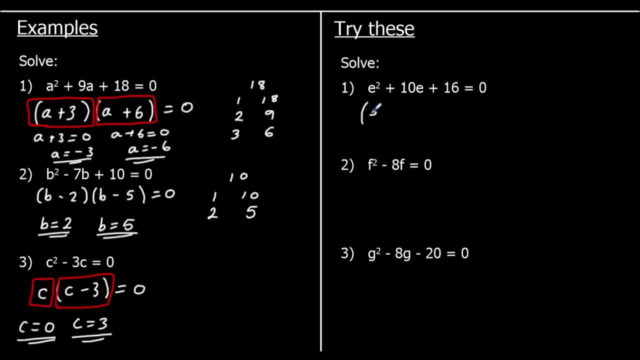 okay. so we've got solve. we're going to factorize and it's a double brackets, so we're looking for what multiplies to make 16. so 1, 16, 2, 8 or 4, 4s, which of those can give me a 10? it's 2 and 8 and it's positive 2. 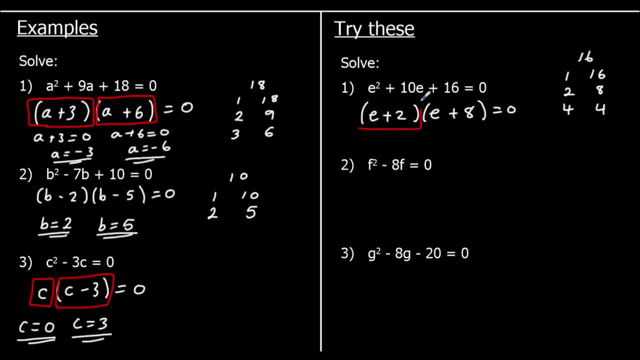 plus 8.. so either e plus 2 is 0 or e plus 8 is 0. so what would e have to be? for the first bracket, negative 2 plus 2 is 0, and for the second bracket, negative 8 plus 8 is 0.. so when we've 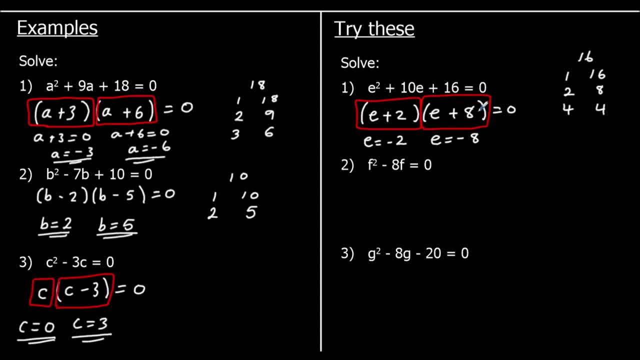 got a plus 2 in the bracket, the answer is negative 2. a plus 8, negative 8.. and for the second one, this is a single bracket, so we're going to take f outside the bracket. f times f makes f squared. f times negative 8 is negative 8 f. so either f equals 0. 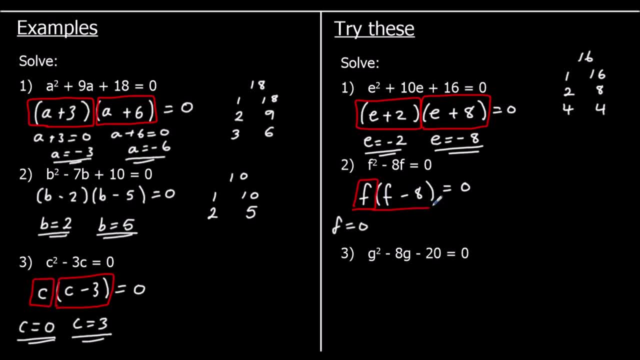 or f minus 8 is 0, and for f minus 8 to be 0, f will do the same. so we're going to do f minus 8 positive 8. and the third one: it's a double bracket G, in both brackets what multiplies to make 20. so we've got 120, two tens or four fives. which of those? 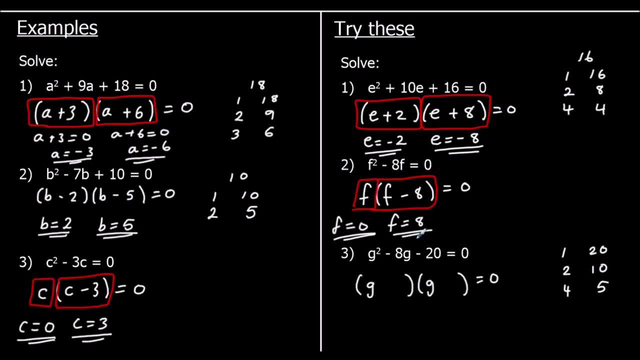 can give me an 8, it's 2 and 10- and we can do plus 2 and take away 10. it doesn't matter if you put them the other way around, you're going to get the same two answers. so either G plus 2 equals 0, which means G must be negative 2, or G. 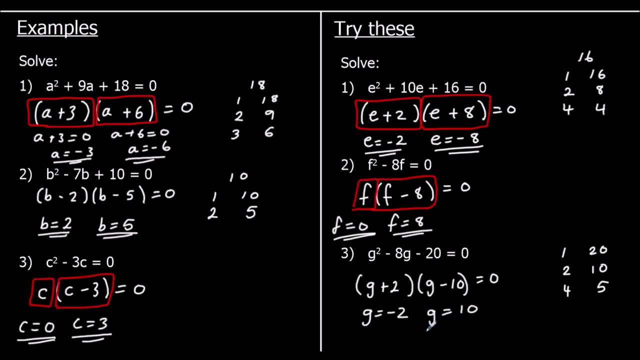 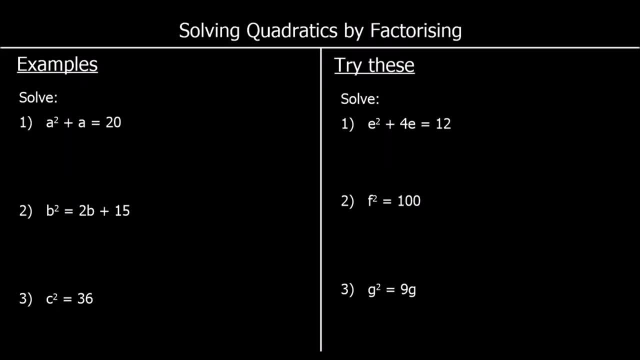 minus 10 equals 0, which would make G 10. here we've got some different questions this time, when we've not been given the questions in the right form. it's not equal to zero, so we need to make it equal to zero before we can solve it. so for the first one, a squared plus a equals 20. 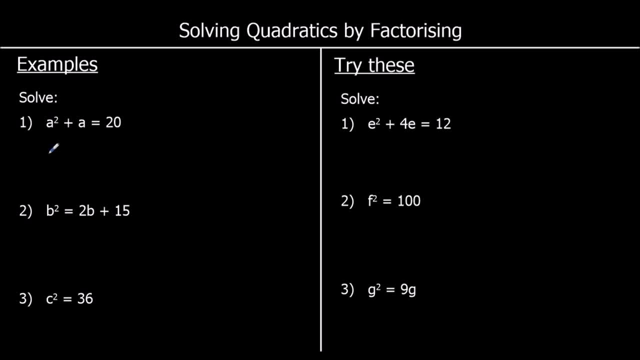 if we take 20 away from both sides, so we'll get a squared plus a equal to zero. so we'll get a squared plus a equals 20. if we take 20 away from both sides, so we'll get a squared plus a minus 20 equals 0.. So now it's equal to 0 and we can solve it by factorizing. 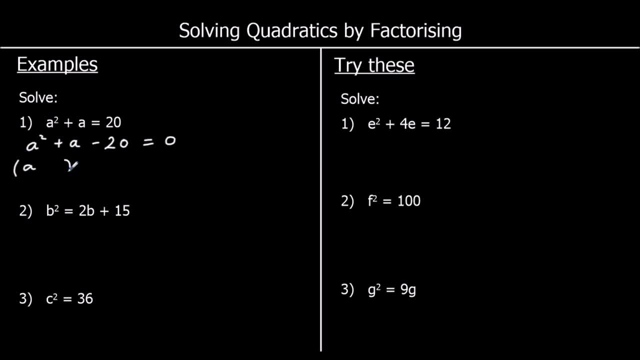 and it's going to be double brackets. What multiplies to make 20? 1, 20,, 2, 10s or 4, 5s? We want to make a plus 1 out of them so we can have a positive 5. take away 4.. 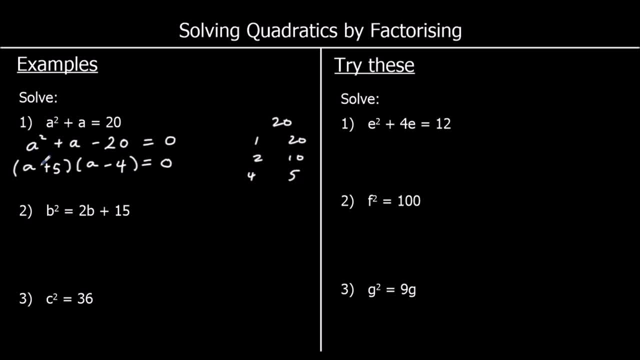 So either the first bracket is equal to 0 or the second bracket is equal to 0.. So for the first bracket to be 0, a would be negative 5, and for the second bracket to be equal to 0, a is positive 4.. 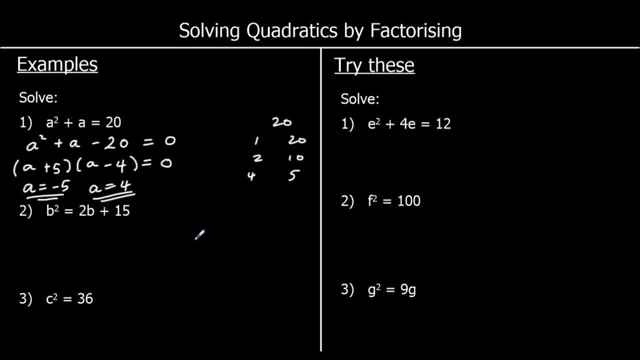 For the second question, again it's not equal to 0, so we need to rearrange it before we can factorize it. So if we take 2b away from both sides and we take 2b away from both sides and take 15 away from both sides, we get it equal to 0.. 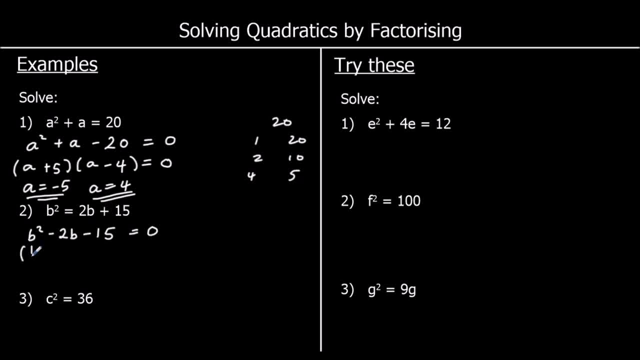 Now we're going to factorize again. it's double brackets. So what multiplies to make 15?? 1, 15 or 3, 5s? We need to make a negative 2, so we'll do plus 3 minus 5.. 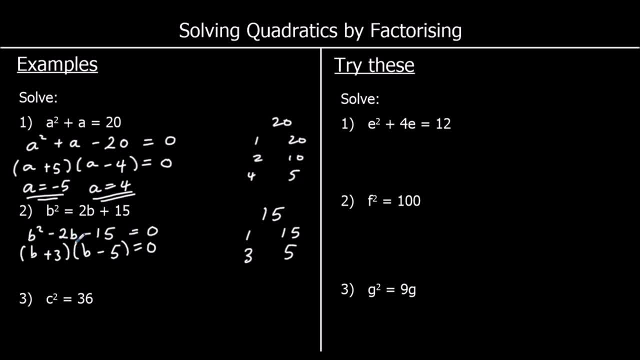 So we take 2b away from both sides and we make a negative 3. So either the first bracket is 0 or the second bracket is 0. so b is negative 3 or b is positive 5.. For number three we've got c, squared equals 36.. 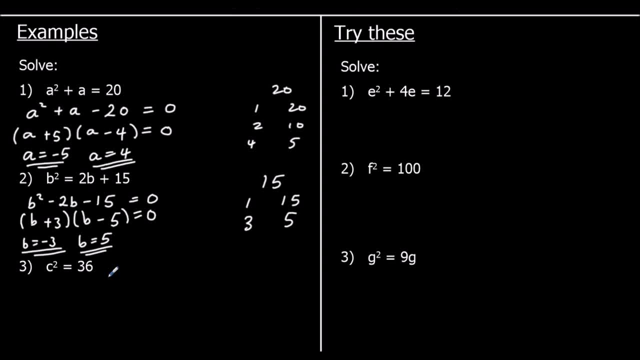 What you could say is: I'm going to do the opposite of squaring, jeg shredding: I'm going to square root both sides. And you could solve it by saying: C is going to be the square root of 36, or what you should say really plus or minus the square root of 36, which is plus or minus 6.. 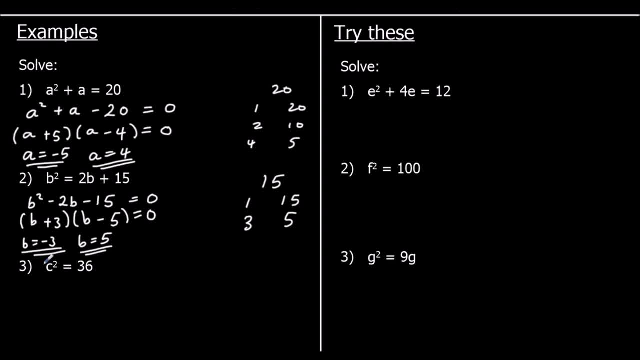 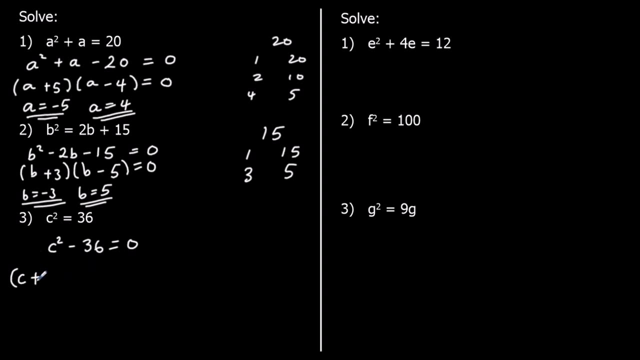 But to solve it by factorising, we're going to subtract 36 from both sides to get it equal to 0. So we've got two squared terms with a minus between them, So it's the difference of two squares. So what multiplies to make 36 and adds to make 0?? 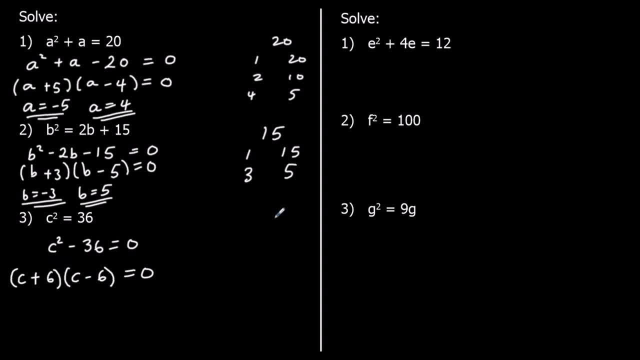 That's plus 6 and minus 6.. So either C plus 6 is equal to 0,, so C is minus 6, or C minus 6 is equal to 0,, so C is positive 6.. OK, three for you to try. 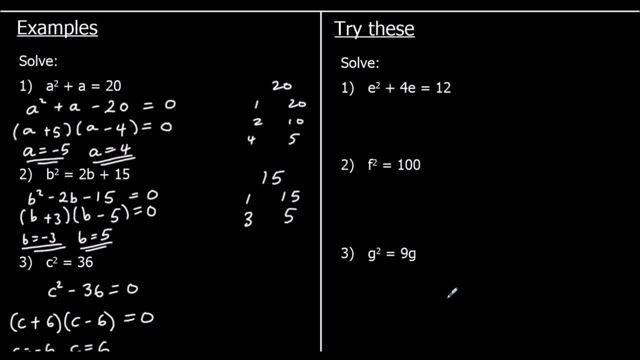 So pause the video. I'm going to give them a go. OK, the first one. we need to subtract 12 from both sides to make it equal to 0 before we start Now we're going to factorise it into double brackets. 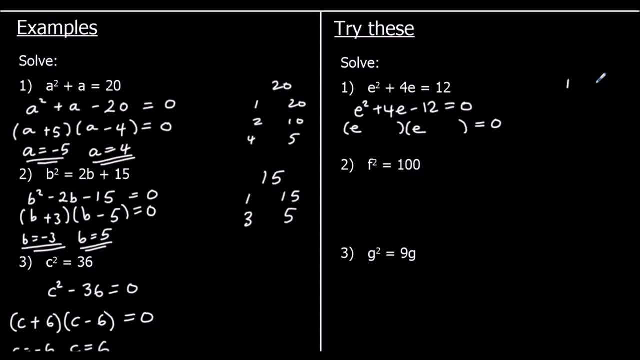 We're going to look for what multiplies to make 12.. So 1 times 12,, 2 times 6, or 3.. 3 times 4. And we need to get a 4, so we're going to have a positive 6 and a negative 2.. 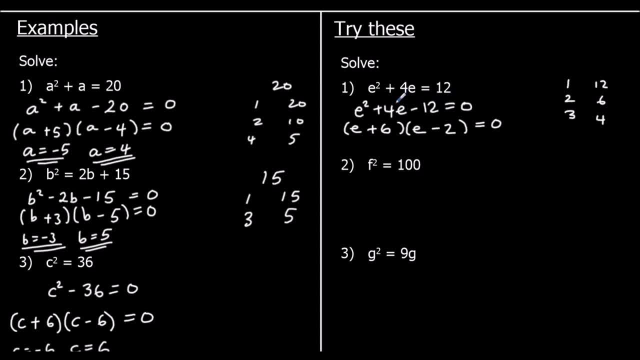 So that multiplies to make negative 12 and adds to make 4.. So either the first bracket is equal to 0 or the second bracket is equal to 0.. So E is negative 6 or positive 2. For the second one we've got F squared equals 100. 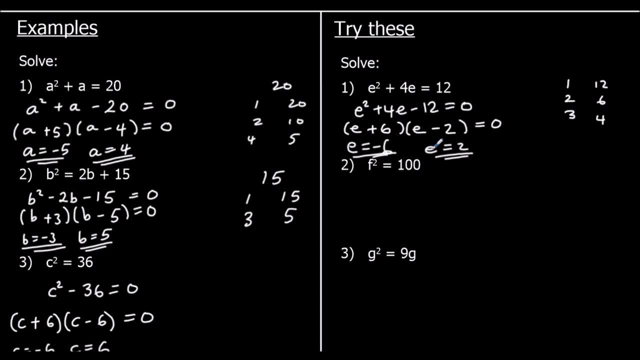 So if we want to factorise it, we could subtract 100 from both sides. Then we'd have F plus 10 and F minus 10.. Or if you don't want to do that, you can say it's plus or minus the square root of 100,. 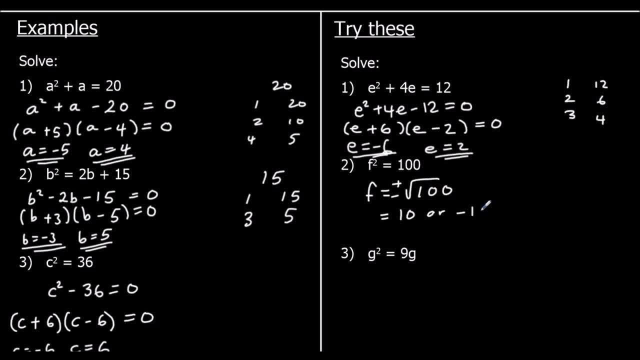 which is 10 or minus 10, negative 10.. And the third one, G squared, equals 9G. OK, So if we want to make it equal to 0 first, so if we take 9G away from both sides, it's equal to 0.. 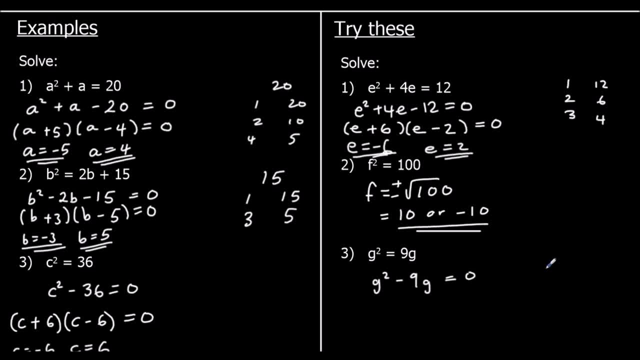 We're going to factorise it. It's a single bracket, single bracket this time. So G outside And G times G is G squared. G times negative 9 is negative 9G. So either G is 0 or G minus 9 is 0, which means G is 9.. 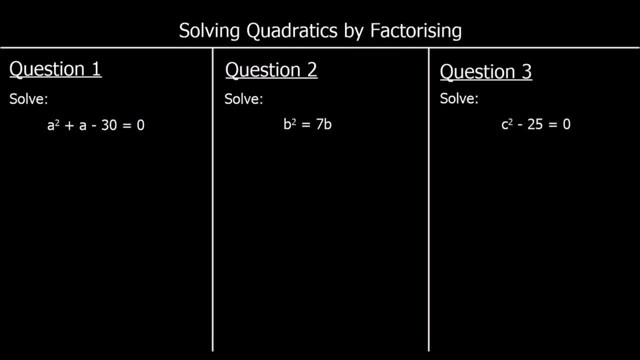 OK, To finish up, we've got three questions, So pause the video, Give them a go. Question one: We're going to have double brackets, so A in both. What multipliers to make 30? 130,, 2, 15s, 3, 10s?